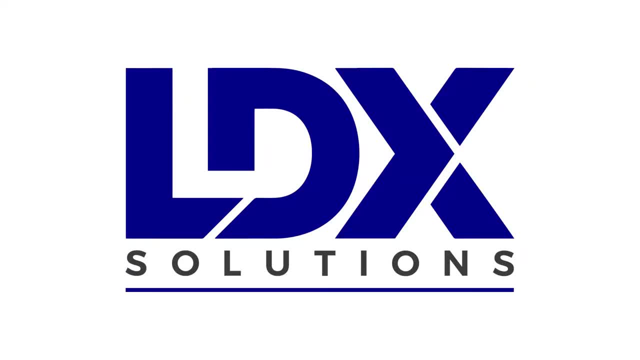 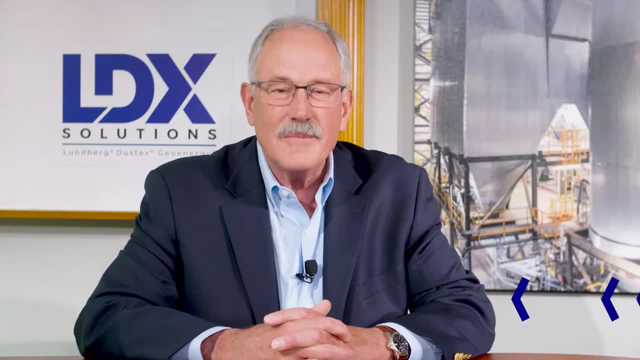 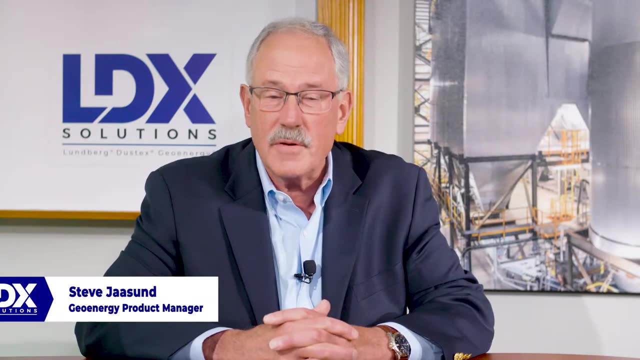 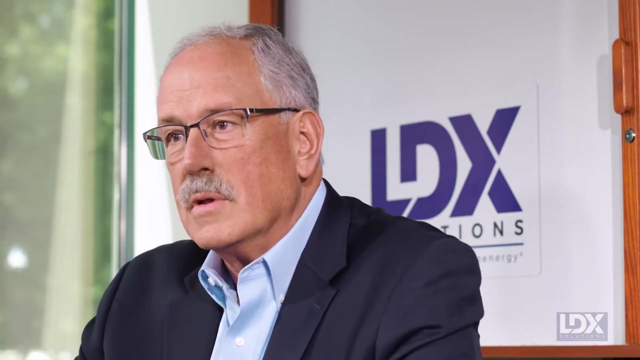 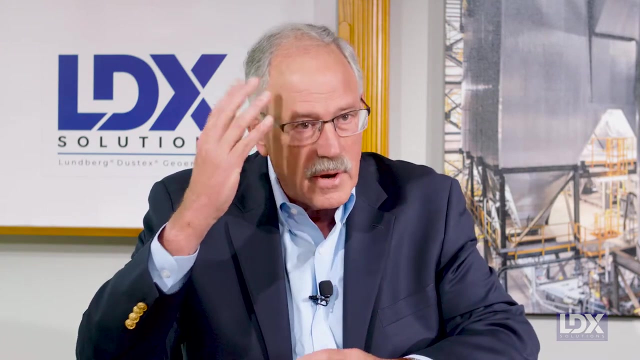 Hello, my name is Steve Jason. I am the geo energy products manager for LDX Solutions, a leading supplier of air quality control systems. We specialize in the development and supply of technologies designed to eliminate air pollution emissions from a wide variety of industrial sources. As you can probably tell from my gray hair, I've been around for a while. 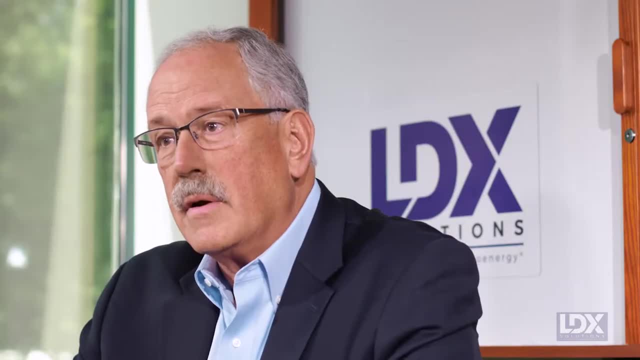 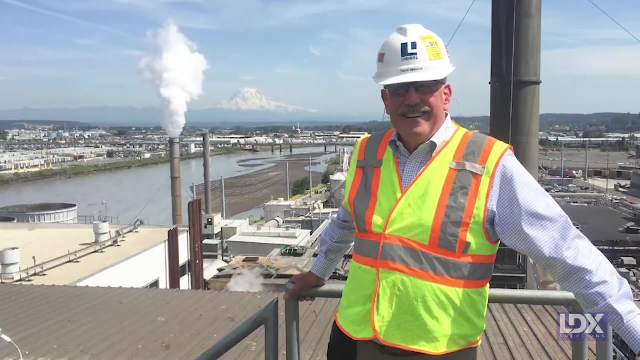 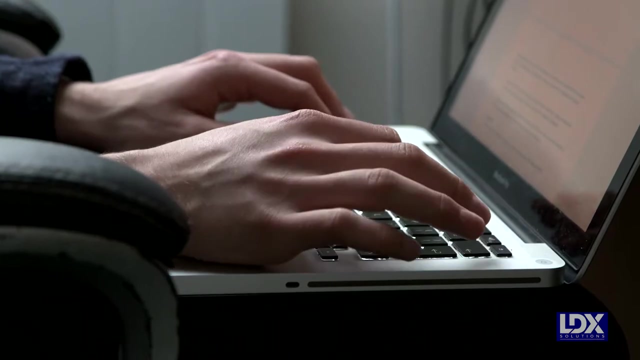 and in fact my entire career has been in the air emission control fields, starting way back in the summer of 1968, the year that marked my decision to jump into my present world. As a young chemical engineering student at Lafayette College, I was wondering what I could. 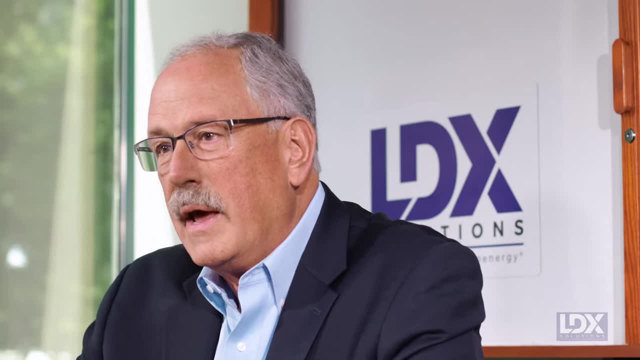 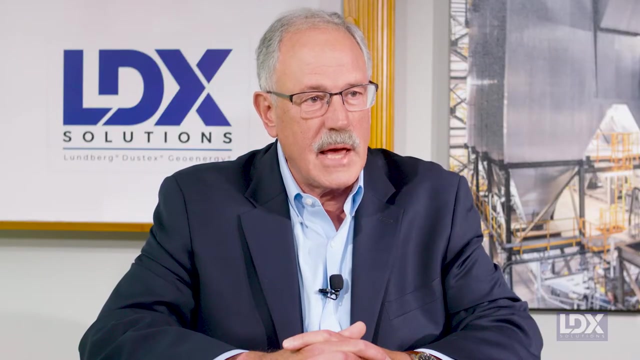 do with a chemical engineering degree. These thoughts weighed heavily on my mind while I was driving home one day on the Garden State Parkway. It was a sweltering July afternoon and I was returning from a fishing trip down at the Jersey Shore. My revelation came about when 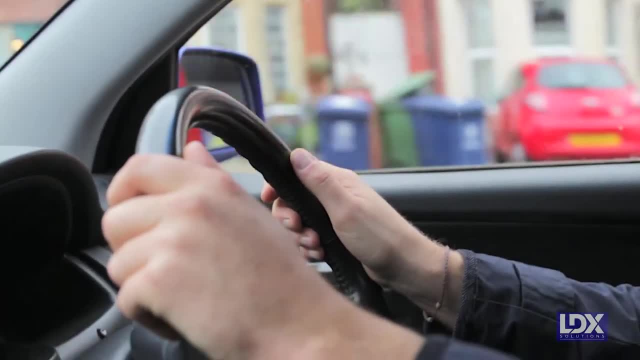 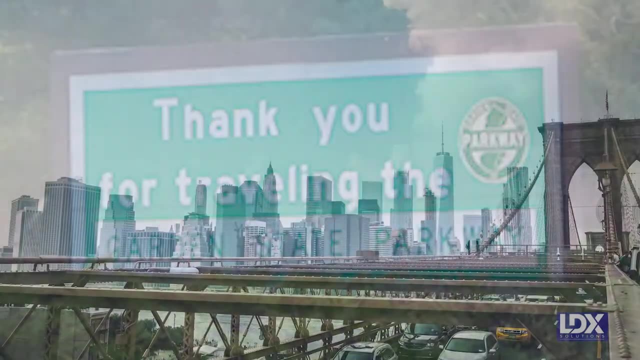 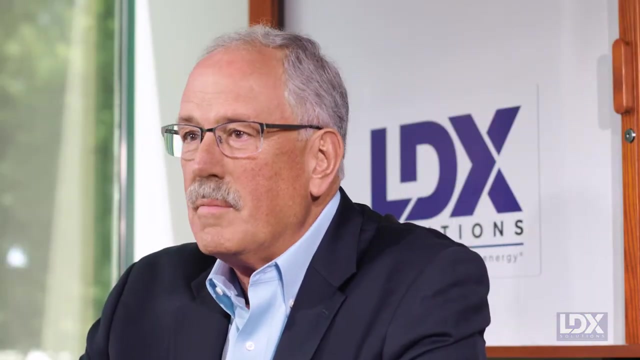 I was stuck in traffic on top of the bridge that spans the Raritan River below. Sitting there in the 90 degree heat, I was choking on the foul air from the myriad factories under the bridge. The foul air was so intense that I remember having to roll up my car windows, despite the 90 degree heat. 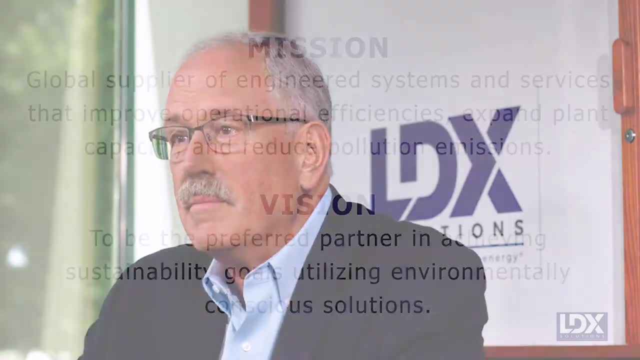 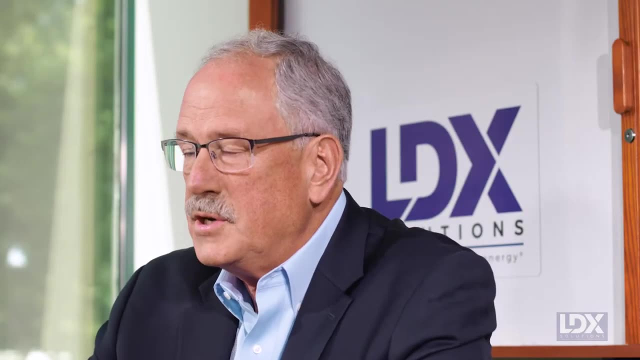 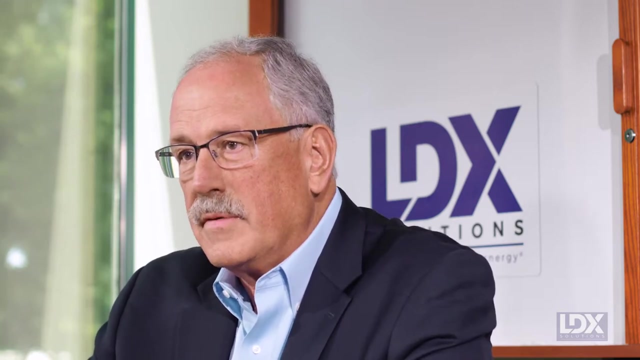 Who had air conditioning in those days? Certainly not me. LDX Solutions' vision is aligned with mine: to be the preferred partner in achieving sustainability goals using environmentally conscious solutions. I am proud to be part of a team of experts that gets us closer to this. 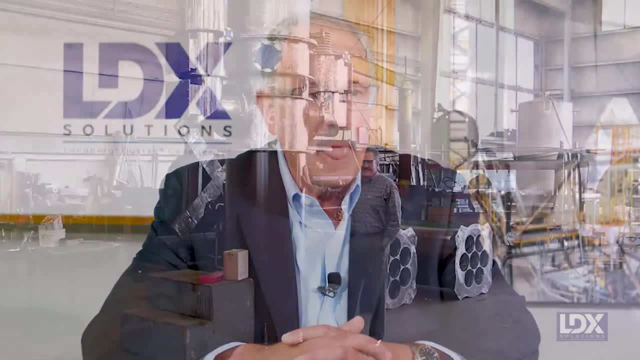 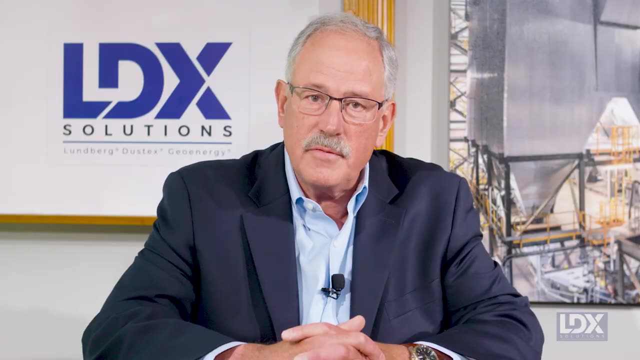 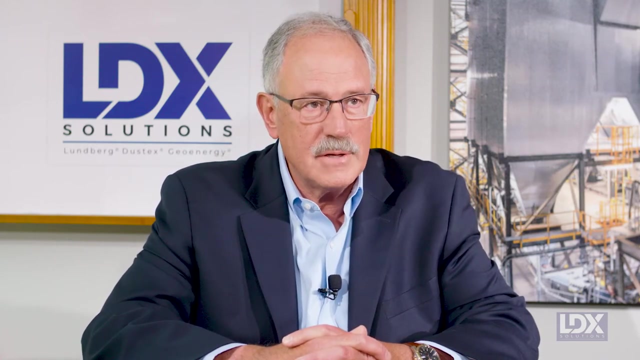 vision every day. Today, our air is much cleaner and I have been a contributor to a healthier planet. How did this happen? What about the future? Here's one man's view Simply stated: the environmental success of the past 50 years has been first motivated by people.